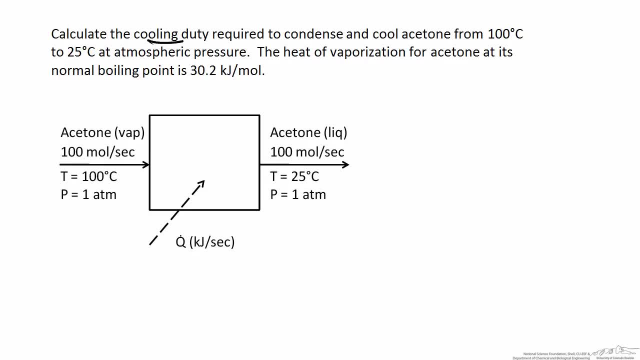 pressure and we know that the heat of vaporization for acetone at its normal boiling point is 30.2 kilojoules per mole. So by definition the normal boiling point is the boiling point at atmospheric pressure. The process is illustrated here in the flow chart below and we can see: 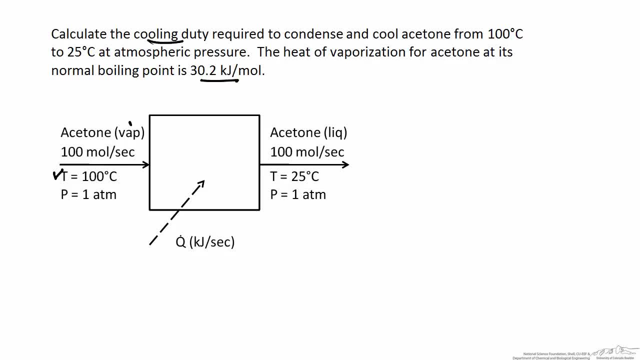 that we have both a change in temperature as well as a change in phase, both of which elicit a change in specific enthalpy, and we're trying to solve for Q. So our open system energy balance- in this case reduces to Q- is equal to delta H, which 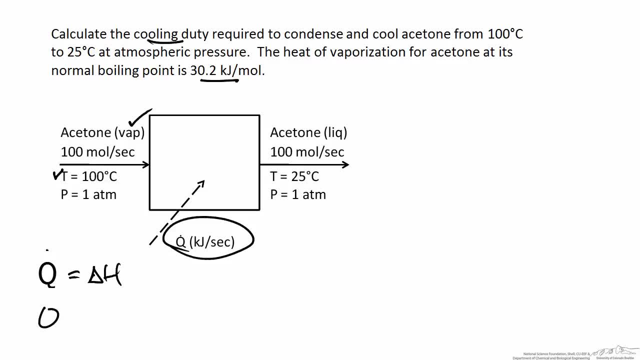 assumes that there's no change in kinetic or potential energy. and we can also write that Q is equal to N dot, which is the molar flow rate times the change in specific enthalpy, which is the enthalpy on a per mole basis. Now, if we had information about the specific 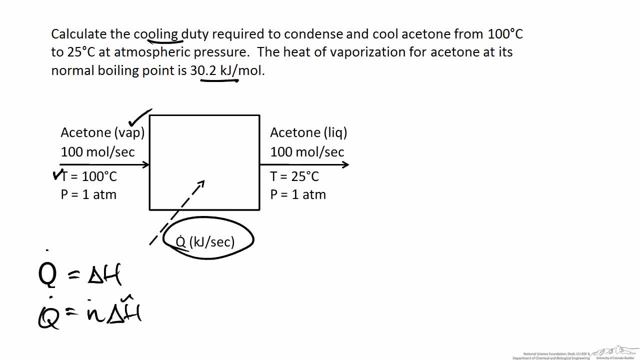 enthalpy of acetone at any temperature and pressure, as we do with water in the case of the steam tables. this would be very easy. We could look up the specific enthalpy of acetone at the outlet, look at the specific enthalpy of acetone at the inlet and take 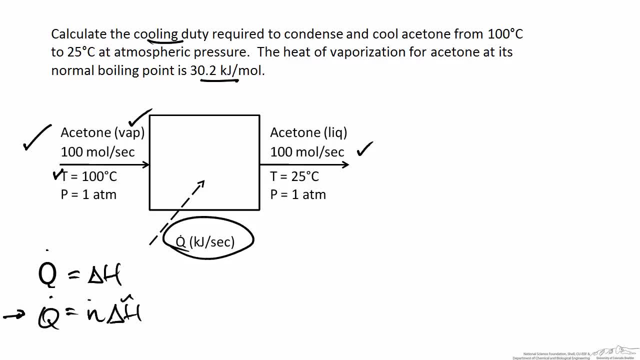 the difference and substitute into our energy balance. Without that information available to us, we have to get more creative and set up a hypothetical path that allows for the calculation of the specific enthalpy for this process. So the key property that allows us to set up a hypothetical path is that enthalpy is a state function, which means that the 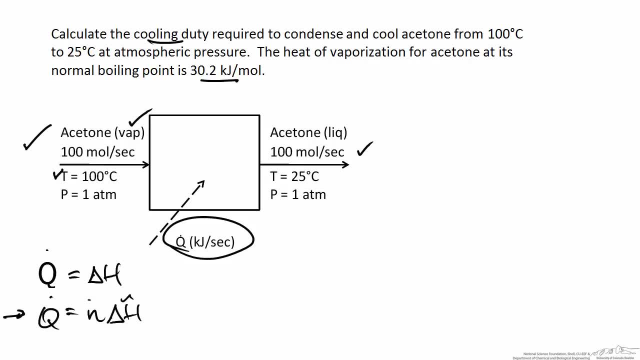 change in enthalpy only depends on the initial and final condition. In this case, our initial condition. we have acetone in the vapor phase, our temperature is 100 degrees C and our pressure is an atmosphere and we are going to the liquid phase at 25 C and we're keeping. 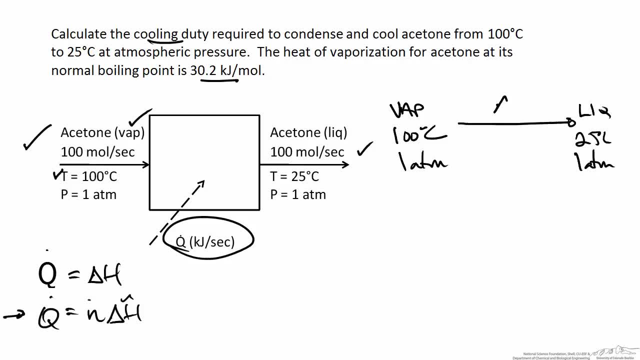 the pressure constant at an atmosphere. So our overall change in enthalpy for the process we can call delta H and we can set up any number of hypothetical steps that's necessary to get from the same initial condition to the final condition. A key piece of information. 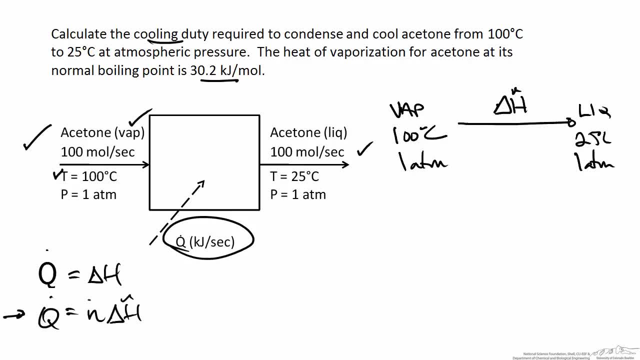 that's going to help us in this process is: what temperature does the phase change occur? We have the heat of vaporization at its normal boiling point, so we need to know what temperature that occurs at In this case, the normal boiling point for acetone is 56 degrees. We could look up this information. 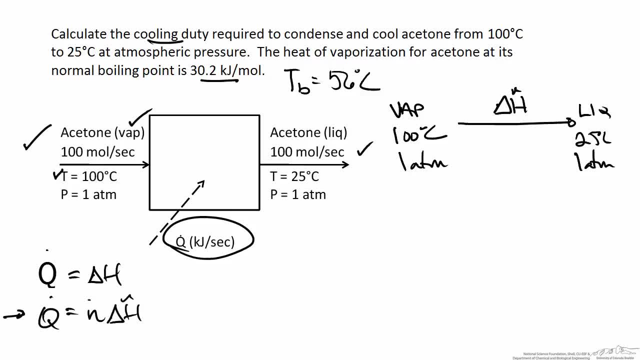 in a variety of different textbooks or chemical engineering handbooks. So we need to get to the temperature at which the phase change occurs. We can get there in one step by changing the temperature and keeping the phase constant. So we have an intermediate temperature, that's. 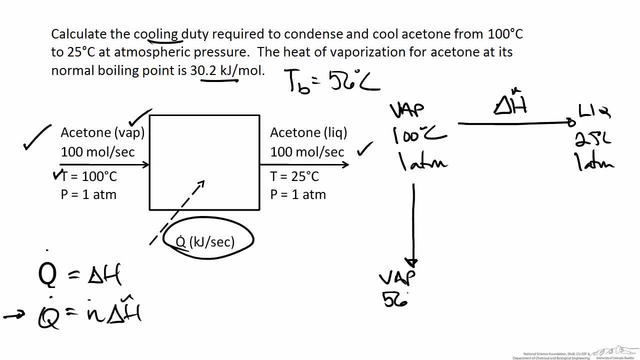 immediate step here, where we have the vapor at the boiling point, which is 56 degrees, and we are keeping the pressure constant in the atmosphere At the boiling point, we are going to change phase. so we have a second step: We are changing phase to the liquid phase. 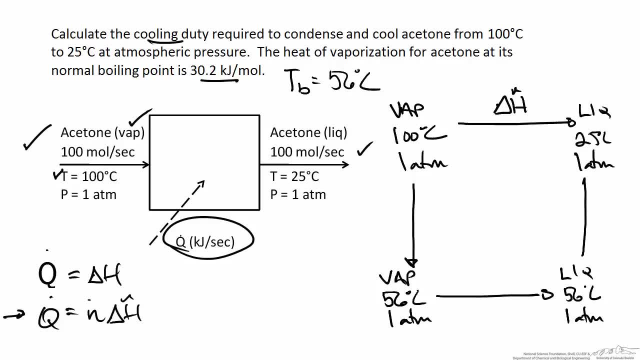 at the same temperature. In our third step we are changing the temperature of the liquid from 56 to 25, while keeping the phase constant. So we have three hypothetical steps here. Each of these has its own change in specific enthalpy, which we will call delta H1,, 2, and. 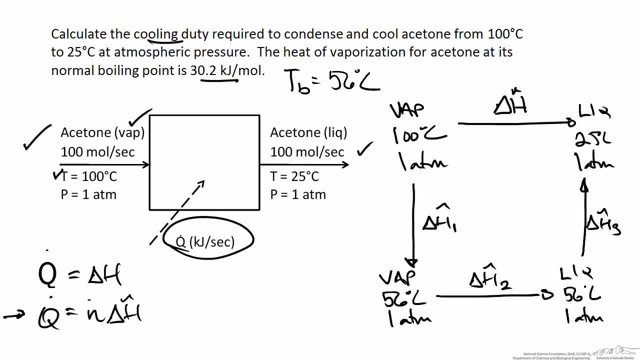 3. And by the definition of the state function, the overall enthalpy here is going to be the sum of these three steps. So we can incorporate that into our energy balance and write that Q is equal to N dot times delta H1 plus delta H2 plus delta H3.. Two of our three steps involve 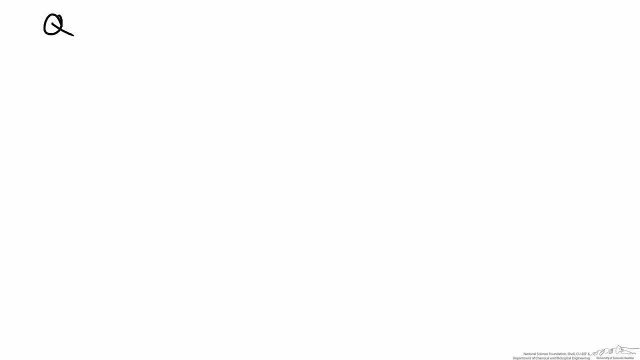 a change in temperature, and any time that we are adding heat and that causes a change in temperature, we are referring to sensible heat. Sensible heat and the change in specific enthalpy associated with sensible heat is related to heat capacity, And so we can calculate a change in specific enthalpy over a specific temperature interval. 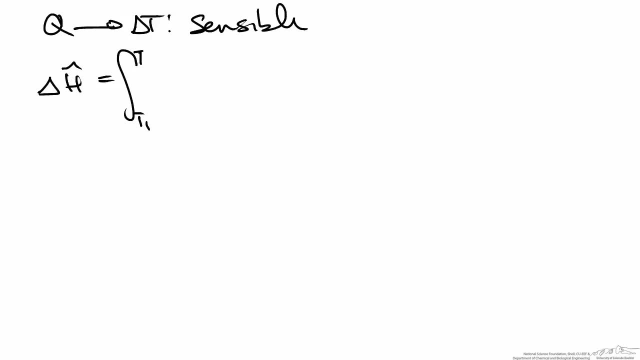 if we integrate over our temperature interval, So from T1 to T2, we integrate the heat capacity, which is a function of temperature, with respect to temperature, And the heat capacity and dependence on temperature is generally expressed as a polynomial function. There are several different polynomial functions that can be used In table B2, in Felder and Rousseau. 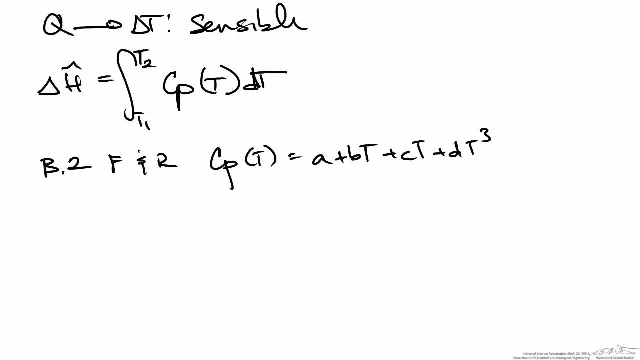 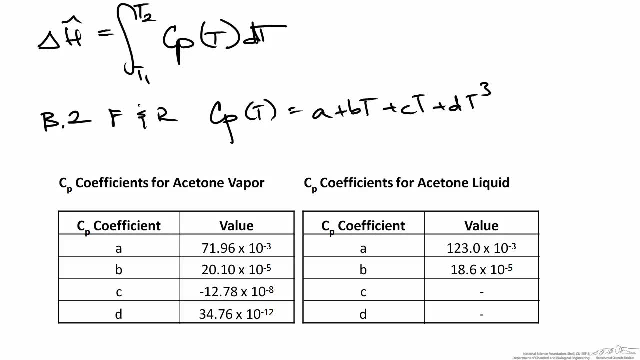 the expression for the heat capacity that is used is so for acetone, we can look up the values for A through D from table B2.. So from table B2 we can see that the coefficients for acetone, vapor and liquid are different. For both the vapor and the liquid, the coefficients 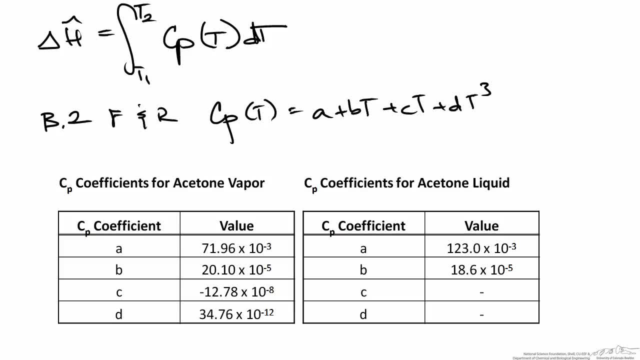 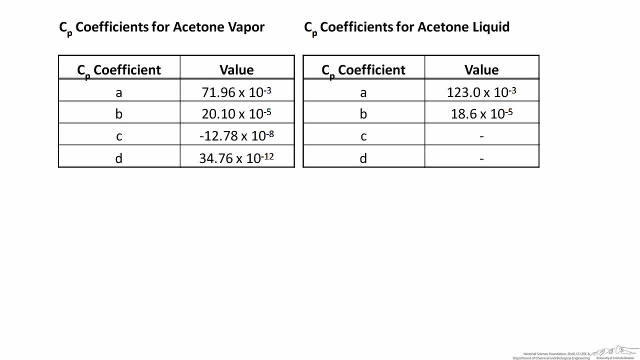 are given in the tables below, which we will use in our sensible heat calculations. In our first step we are cooling acetone vapor from the inlet condition at 100 to the boiling point. So we can calculate delta H1 by integrating from 100 to the boiling. 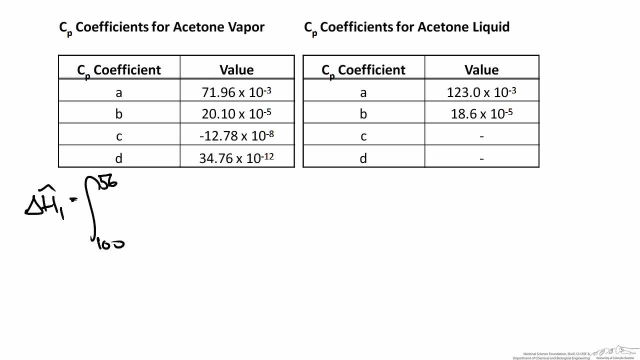 point at 56, the heat capacity, where we have four coefficients. If we evaluate this integral and plug in our coefficients and limits of integration, we will find that the sensible heat associated with this process is negative 3.82 kilojoules per mole. Our second step. 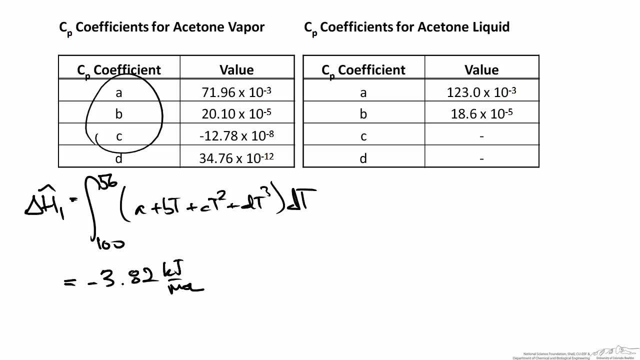 involved a change in phase. So we are going to look at the heat capacity of acetone vapor from table B2.. So our first step is to integrate the heat capacity from the boiling point at 56 to the outlet condition at 25.. And here we have two coefficients. So we are integrating. 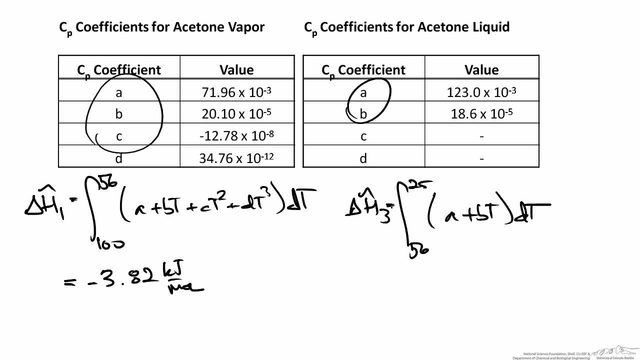 A plus BT with respect to temperature, And if we evaluate this integral and plug in the coefficients, we find that the sensible heat for this step is negative 4.06 kilojoules per mole. The last change in enthalpy that we need to calculate is delta H2, which is associated. 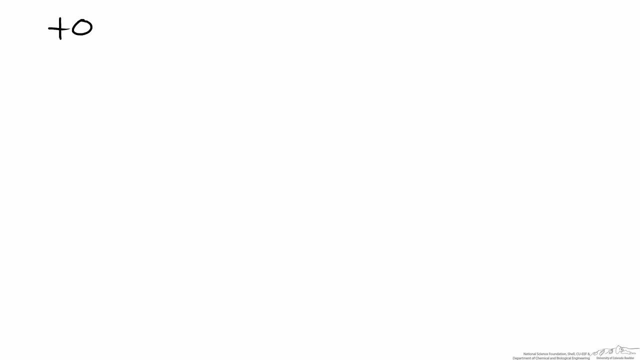 with a change in phase. Any time that we're adding heat and we're changing phase, we're referring to latent heat. We know some information about the phase change and the heat that is absorbed when acetone is vaporized at the boiling point. In the beginning we were given the heat of vaporization is 30.2 kilojoules per mole and 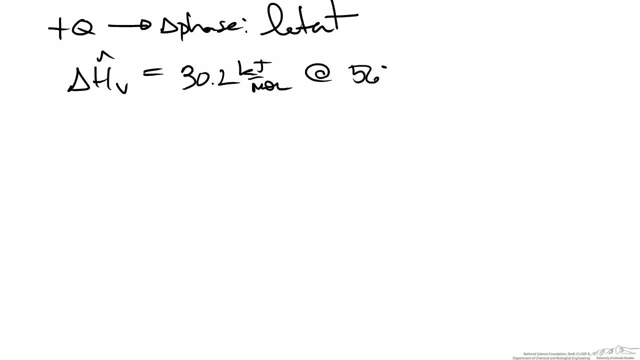 that is specifically at the normal boiling point at 56 degrees in an atmosphere of pressure. So in this case we are condensing, we are not vaporizing, but we can still use this information if we consider that enthalpy is a state function. 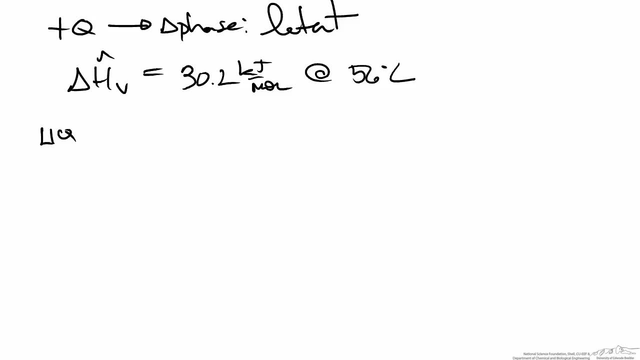 If we consider the path, the heat of vaporization represents the transition from a liquid to a vapor and a state function, by definition, only depends on the initial and final condition. So if we reverse our final and initial condition And we consider our path, In this case, to be the transition from a vapor to a liquid, then the change in enthalpy associated